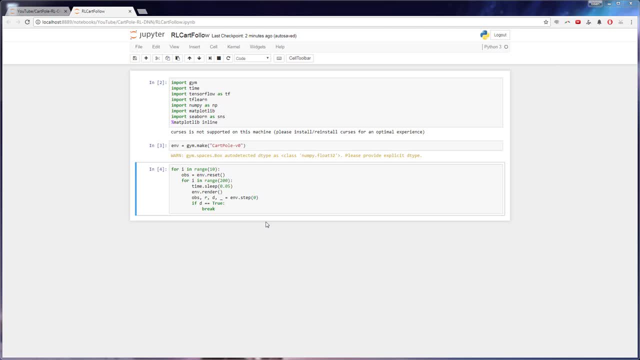 To the way we would approach any supervised learning problem. we'll have an input, we will have a few layers- In this case we're going to be using normal fully connected feed forward layers- And then we'll have a loss and we'll try to optimize that loss and minimize 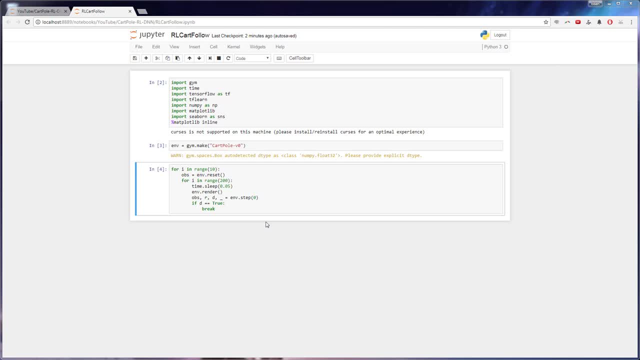 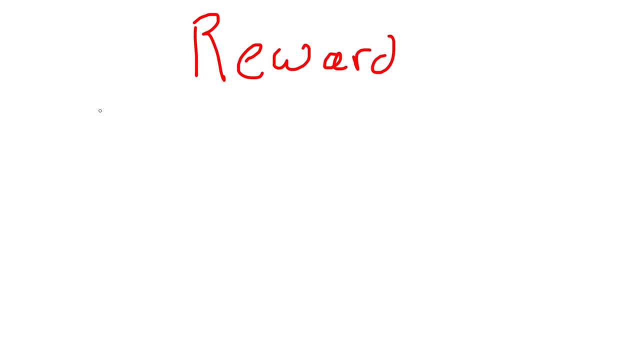 that loss. So what's the difference? And the real difference is is that, instead of our loss being calculated by how wrong we were, our loss is actually decided by what our reward is. So if we have a positive, a lot of positive rewards and we're doing well, well then our loss. 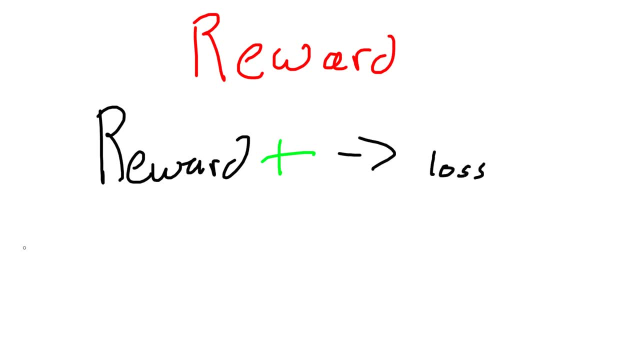 is going to be pretty small. right, Because we're not doing anything too wrong. But if we have a lot of negative reward- which in the cart pull example, won't be the case, but if we did have a lot of negative reward, our loss would be very, very high because we would have a lot of error. So 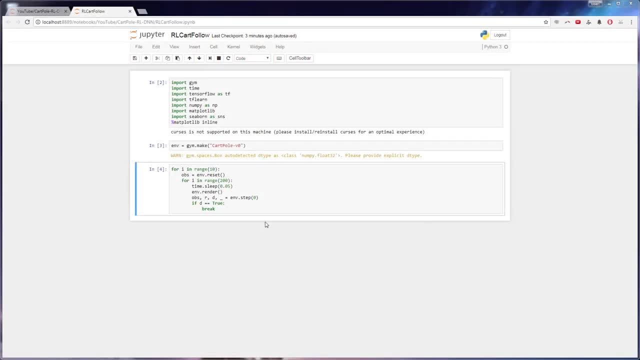 all we're going to do is build out that normal, that neural network like normal, but our error will. our error will be very high, So we're going to have a lot of error. Our loss will be calculated using our reward. So, jumping into that, I'm actually going to create. 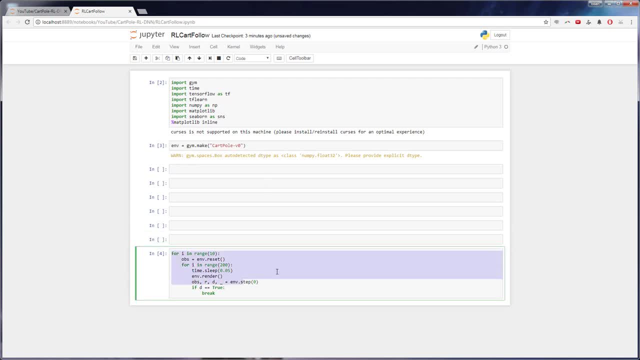 a few cells right here. We'll come back to this later, after we've got our network made. So the first thing we want is we want an input layer, and I'm going to be using TF learn. So if you don't know TF learn- I also have a video on that. It's pretty simple. Lots of this will also. 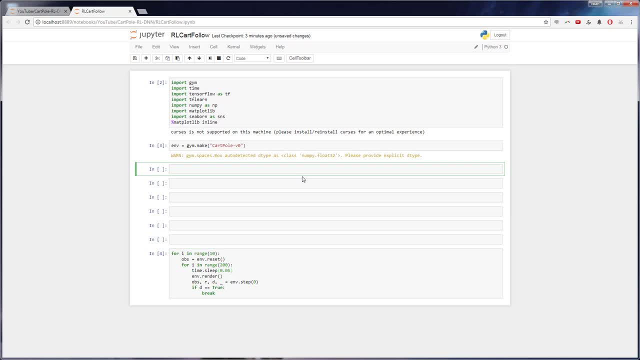 just be normal TensorFlow. So the first thing we need is an input, is something for input data. So we'll call that an input layer, And then we're going to use an input layer, And then we're going to use an input layer, And then we're going to use an input layer, And then we're going to have. 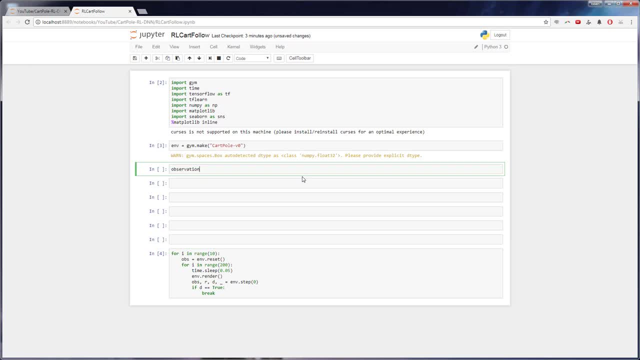 the observation. observation right, Because the observation is what we get from our environment, So our observation. remember earlier, if we printed out the environment, we got four different values for the state of the game, So we'll create input value for as many frames as we want in four. 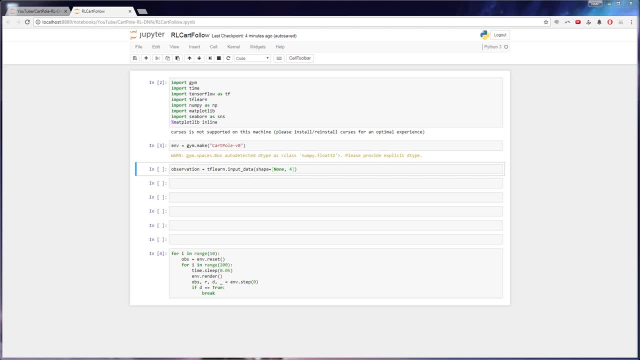 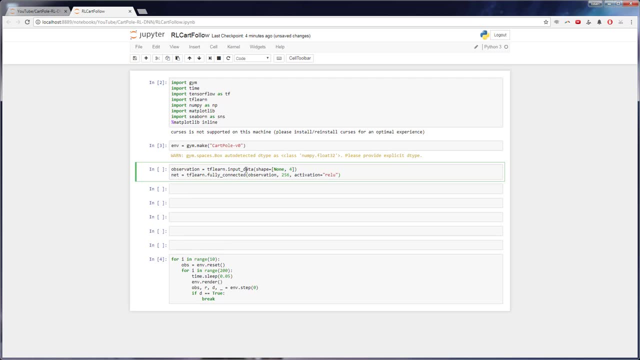 values. Next, what we'll go ahead and do is we will start making our actual dense layers. So we'll start off by creating a network and having a framework for that And then we'll go ahead and fully connected layer from the input data to this, or rather, we'll connect the input layer. 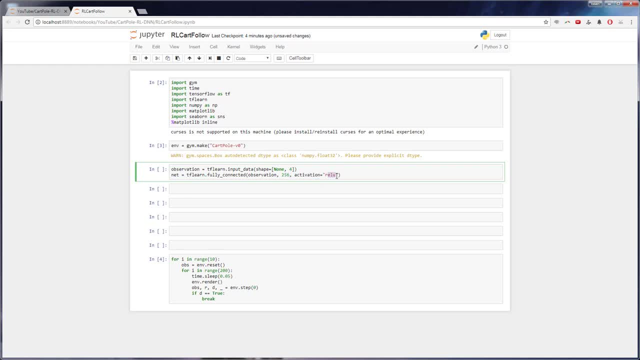 to a new layer with 256 nodes and a relu activation function. Now, there's a thousand ways you can do this, but I'm just going to do it this way. So there's a lot of questions you can ask, and some of them I'll be able to answer, as to why I made certain choices, but some of them are just because. 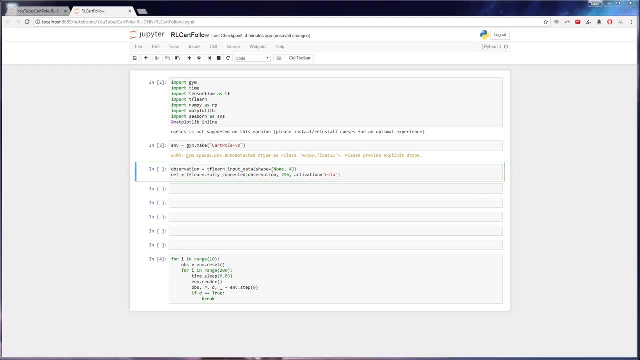 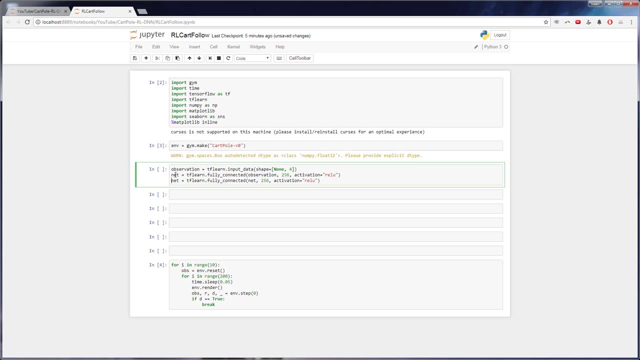 they work. Other ways might honestly work better. So we're going to do this same thing two more times and just have a few layers. The only difference in this layer is that we're connecting another layer to this network, not the input data, So make sure to change this right here. 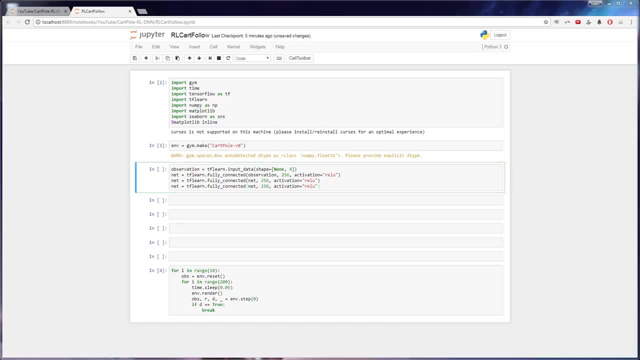 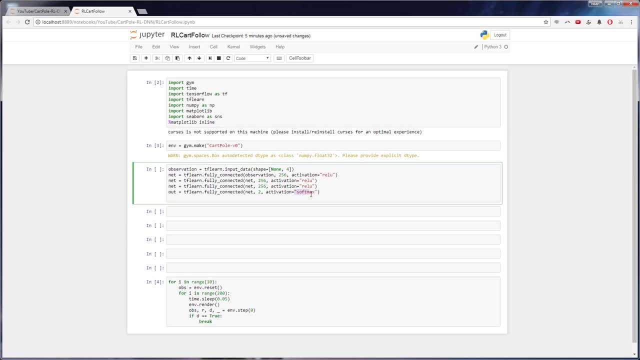 Awesome. So we have three densely connected layers and then we're going to want to finish that out with a output layer that has two nodes, one for left and one for right, and uses a soft max. And the reason we use soft max is because we want the probability. or rather, yeah, I guess not. 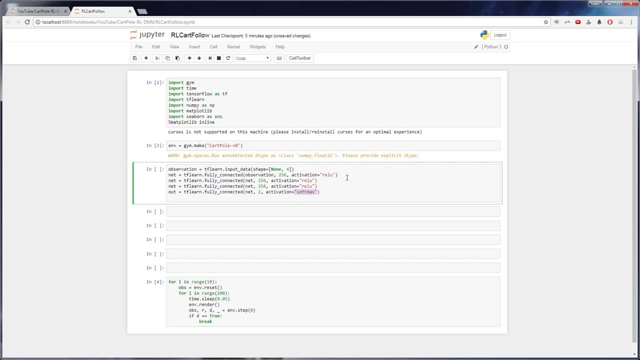 necessarily the probability, but the likelihood That going left will be what we want and the likelihood that going right will be what we want- Awesome. So now that we've got that, here's where things start to get a little different, right. 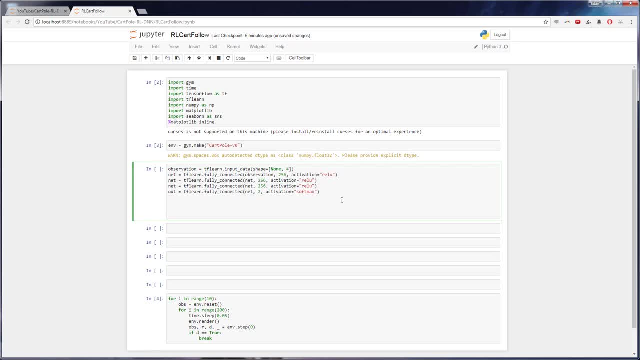 Because to be able to process what our law should be, we need to know what action we took and how much reward we got for taking that action. So for the reward, we'll type out, we'll call it reward holder and we'll say it's equal to tfplaceholder And this placeholder will be a float. 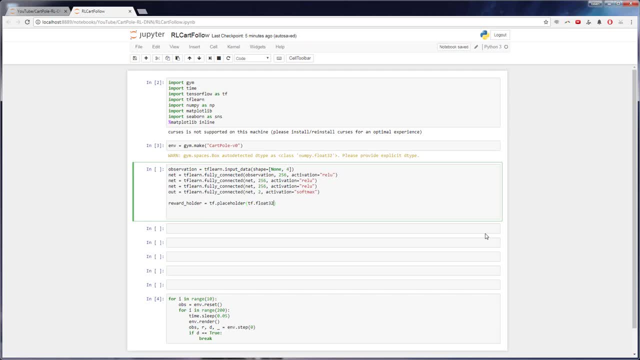 Because our- as you might guess, our- reward can be any number. Well, I mean, in Carpool it's always going to be one or nothing, But in other cases we might have floats, and this works as a float too. 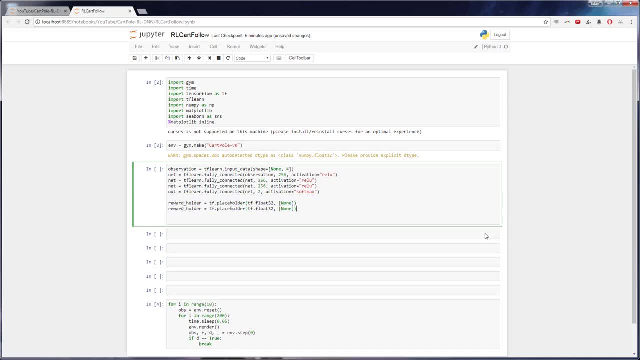 And we can have just as many as we have frames, so no specific dimensioning. And then we'll want something similar, but an action holder which will tell us which action we took. So for the action holder, we're actually going to have an int And there's different ways you could represent. 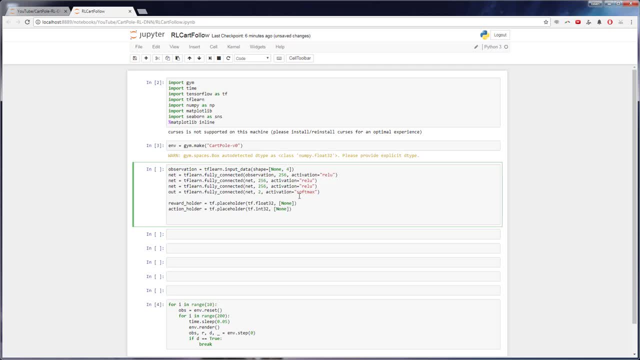 this. But once we actually get into how I'm going to do this, we're going to have an int And then, once we do it, you'll see why we need an int here soon. So what we actually want to do is: you got. 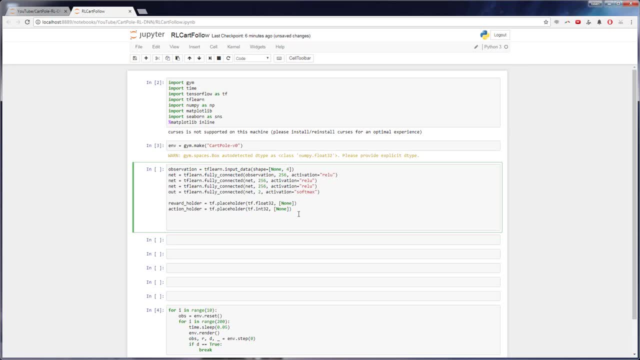 to keep in mind right when we pass our observations through our neural network and get out a result or an output. only one of our- to some extent you can say- only one of the two nodes, one of the two output nodes, is at fault, Because if we went to, if we went left when we should have gone, 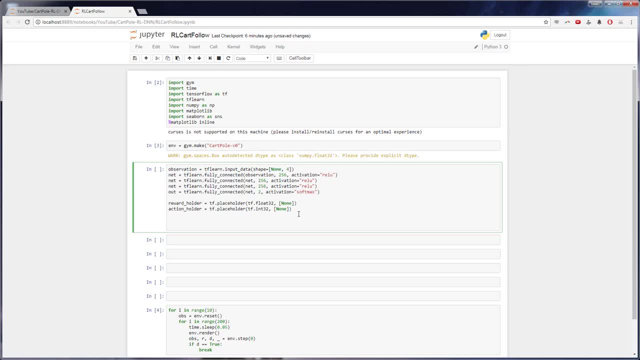 right. well then our left node was too strong. Technically you could also say the right one was too weak. But the way the math kind of works out for us is that if we say the left one was too strong, well, we kind of want to take that, make sure that one's responsible and adjust it. 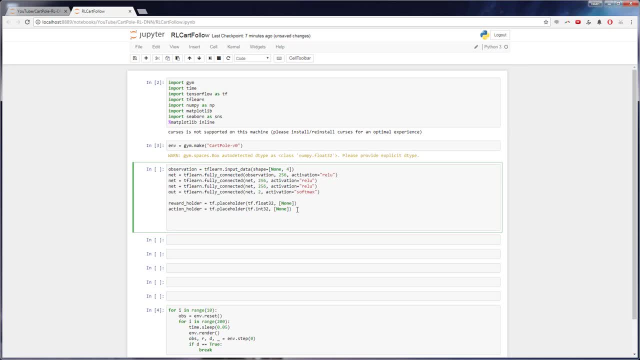 accordingly. not everything, just the nodes that were wrong. So to get the responsible outputs, this is a little bit tricky right? But follow with me, I'll try to explain it as best as I can. So we'll say responsible output. 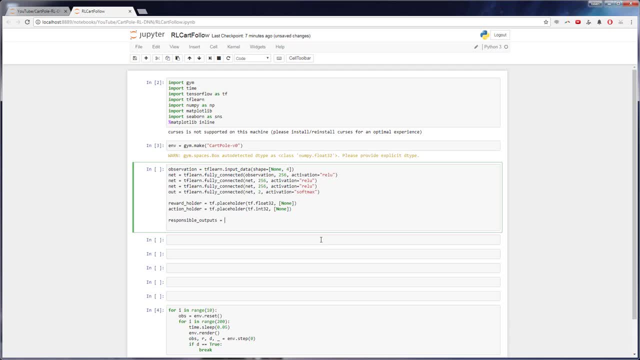 I mean honestly, yeah, outputs, And what we're going to do is we're going to gather the nodes, So tf dot gather. I'm going to write this out really quick and then kind of explain it as I go. So the first: 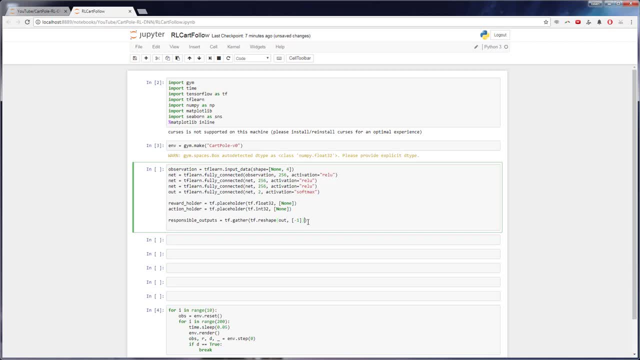 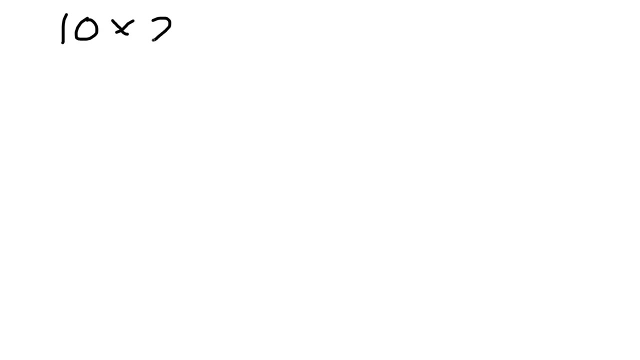 thing we want to do is take all the nodes in our output layer, right? So if we do tf dot reshape out to negative one, this is just taking all of the outputs from every frame, right? So let's say we have 10 frames. each of those frames has two possible outputs. So that's just you know. 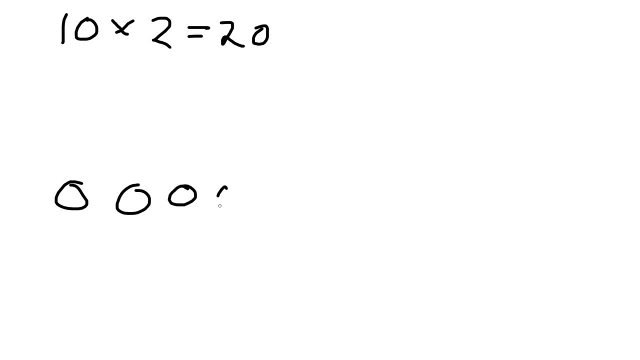 20 output nodes, right. So we're reshaping those all and we're kind of flattening them. And then what we want to do is, from each of those nodes we want to get the one which action we took- And by that I mean for the first two nodes in this giant flattened list- if we went left. 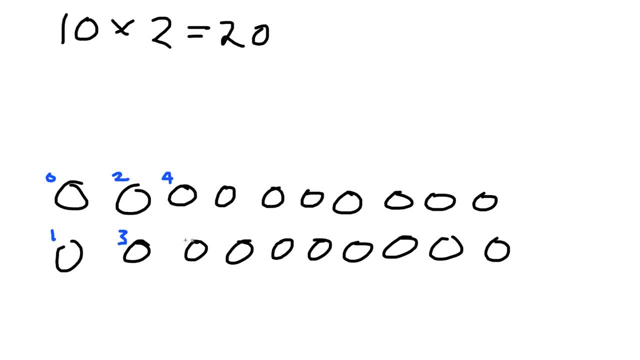 we want to get the first node. if we want went right, we want to get the second node. Now for the second frame, we're going to have the third and fourth output nodes. If we took a left, we'll want the third node, if we took a right, we'll want the fourth node And essentially the. 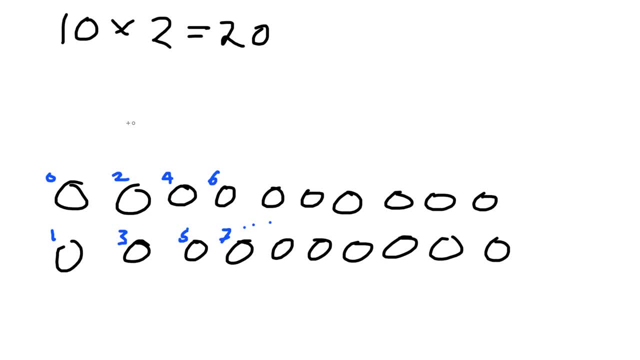 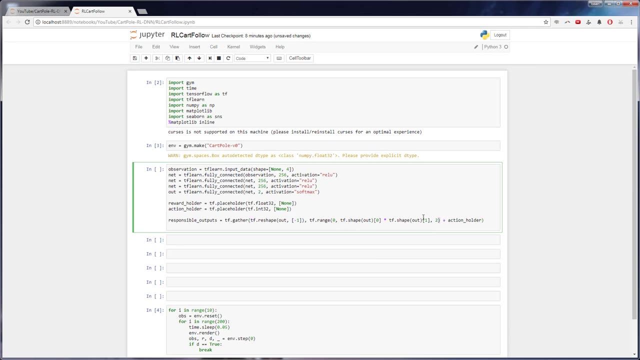 way we do this is with tf gather. So from these, the ones we want to gather are- and there's a little again, there's a little bit tricky here, but stick with me As I go through this. what we'll want is this right here. So what we're doing is taking it step by step. 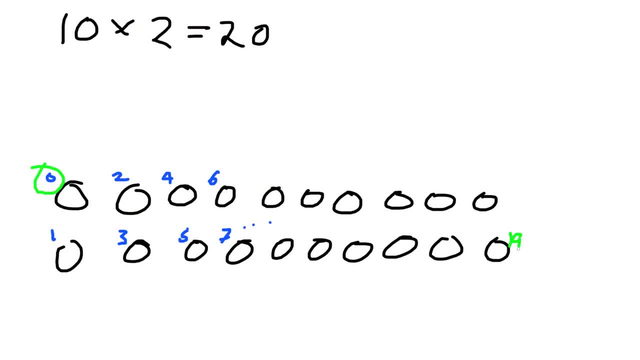 is we take a range right. Our range is from zero to the total amount of nodes we have. This is the total amount of nodes we have. There's, let's say, 10 frames, two nodes in each frame, So that would be 20 nodes. And we want to increment this range by two at a time, So we'll have 0246.. 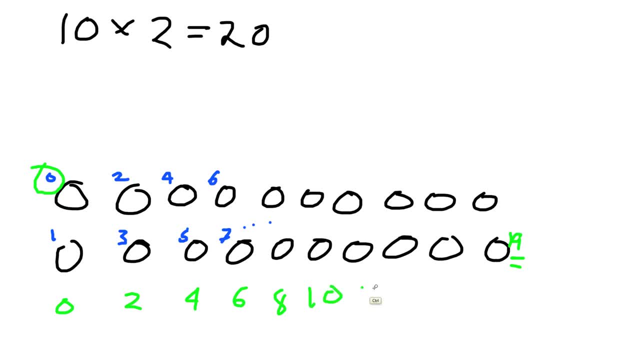 And so on all the way up to 20, or not 2018,, I guess- And then we'll add the action holder. So what this does is, if we have a list, say 0246, and so on, and the first node, we take a left. 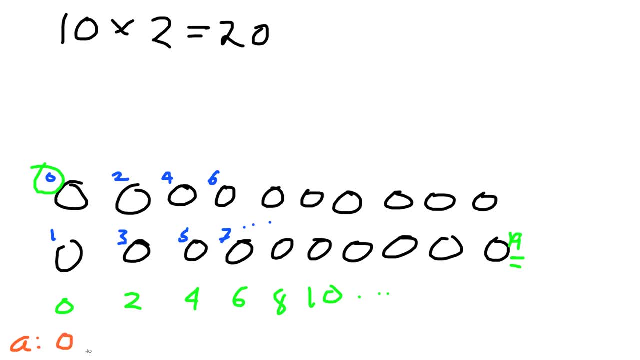 left. well, the action is a zero right because we have an action that's zero or one. so if we take a left, well, we start at zero, we add zero for our action, we end up at zero. so we're taking the first node, which is a left. now let's say we have the maybe fifth node right, or we're talking about the 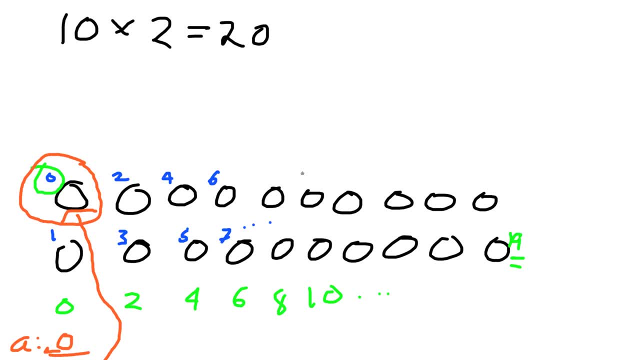 fifth frame. so the fifth frame uses the nodes, the 10 and the 11th nodes. so we start off at 10 or 11, and then our action is either zero or one. so if we take zero, 10 plus zero is, as my guess, 10, that's. 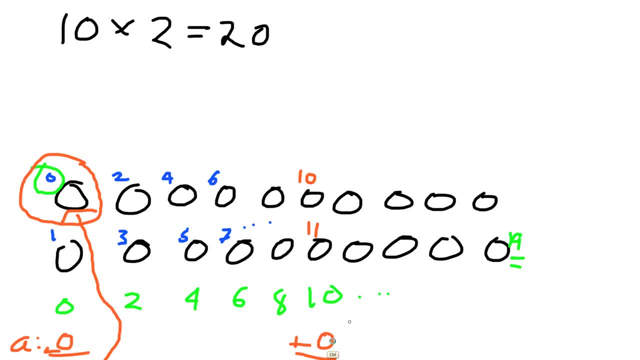 a left, and if we have, if we have a right, that would be a one action, the action would be a one. so 10 plus 1 is 11, and 11 was the node that represents the right movement. now this is the definitely the most complicated weird thing in the entire tutorial. so if you don't get it right, 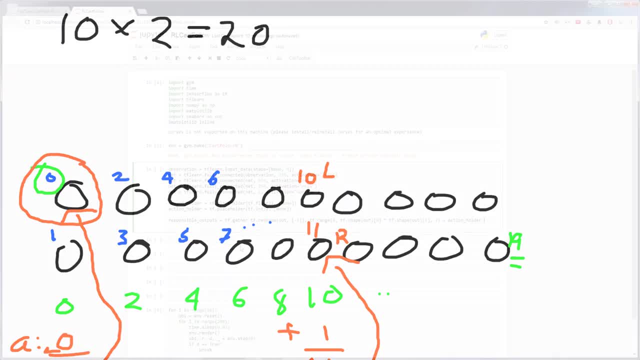 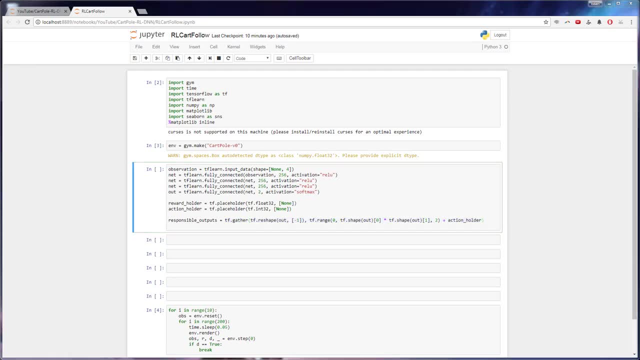 away. it took me forever to understand this. just go over it. if you times, experiment with kind of how this works and think over it a few times, and once you get this, you're definitely going to get everything else, no problem. so moving on, now we can calculate. 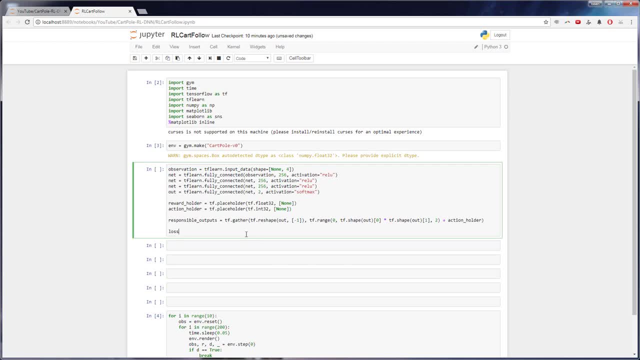 our loss now that we know which outputs are responsible, so you can say the loss is equal to negative. and this is very similar to what we've done in the past: tf-dot reducing, reduce and then from here we want to log, and this is again very standard way of taking loss. 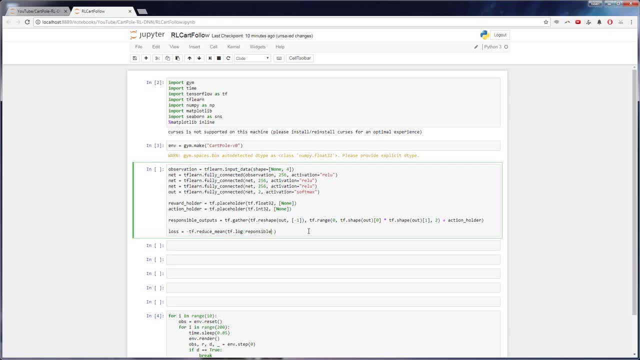 and log our responsible outputs, responsible outputs- and then we want to multiply that by the reward holder. and why do we do that? the reason we do that is because we want our loss to be kind of corresponding to our reward. so let's say we got a negative 10 reward, right? um well, we want. 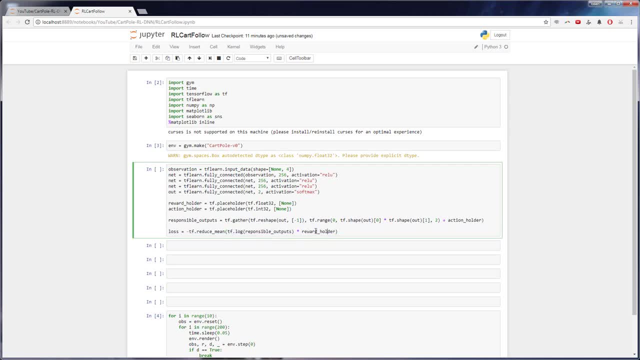 our loss. this part right here to be negative. so multiplying our reward by our actual outputs that were wrong tells us it kind of changes the scale and magnitude of our loss, which is, i mean, what the reward should be right. our reward is what decides how much loss we have, and then we just need to 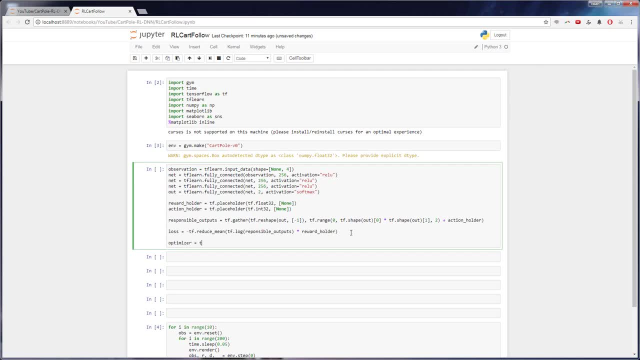 make you know a nice optimizer, um, simple, the standard stuff. right here we're going to use an atom optimizer. there's other things you can use. i'm just using this because it works, um, and for our update step. what we're going to do is we are going to have that optimizer minimize our minimize. 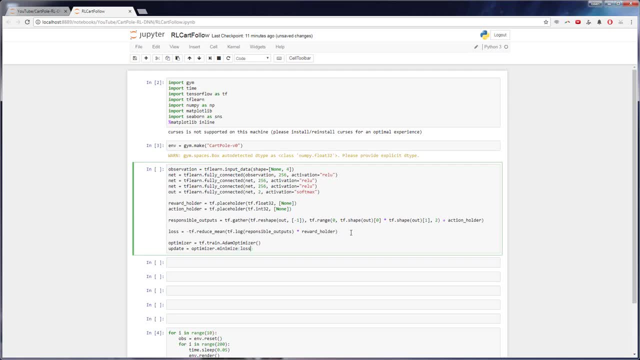 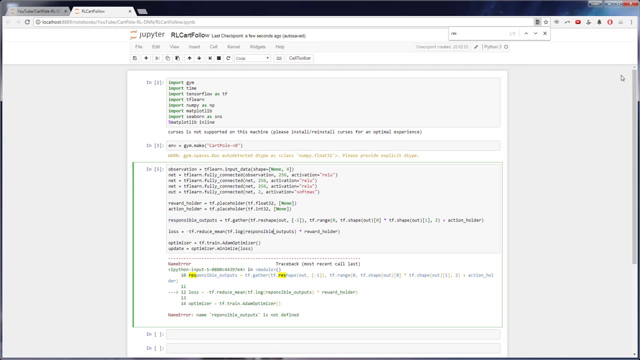 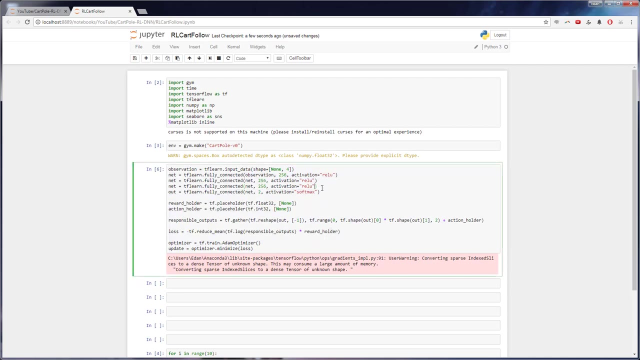 minimize, minimize, yeah, minimize our loss. so hopefully, no error is there? oh, responsible outputs- where is that? responsible outputs? cool, hopefully, that's good there, awesome. so we've got our actual model built- by far, i think, the hardest part right here. so if you've made it this part, especially past this line, you're doing pretty good. thank you guys. 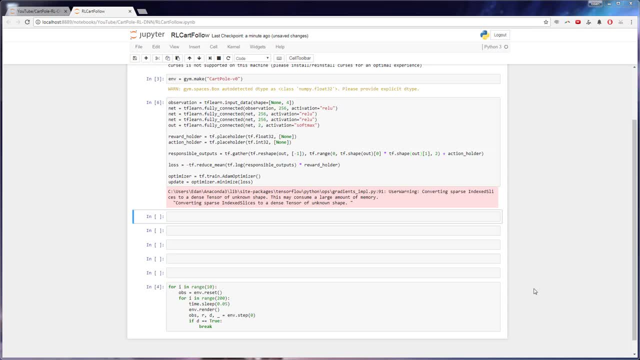 so much for joining me for this tutorial. i hope you guys. i know it was confusing and we don't have to show yet, but definitely stick in for the next tutorial or two where we finish this up and actually see the fruits of this labor, because this neural network right here i know it's pretty. 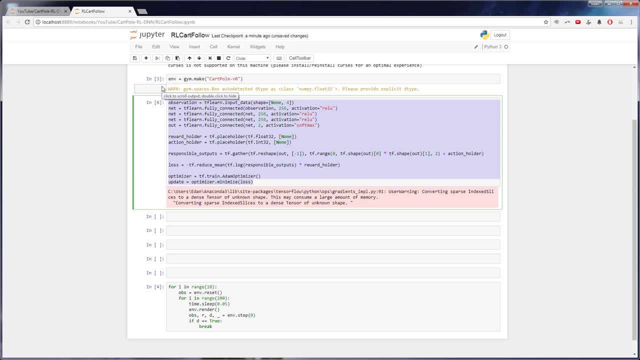 complex, but it will get us some pretty cool results. so thank you for sticking around till the end. if this video helped you out, i really appreciate it. if you consider leaving a like and subscribing. definitely check out the next videos and i'll see you guys next time. thank you.